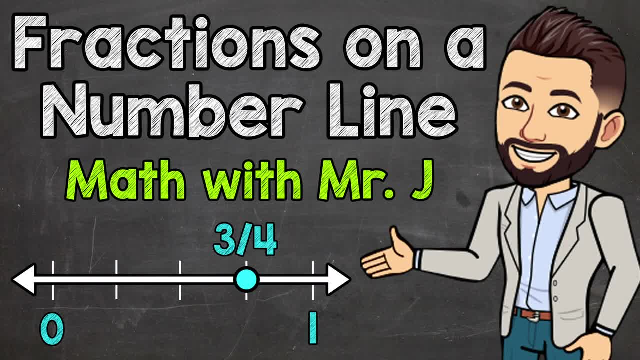 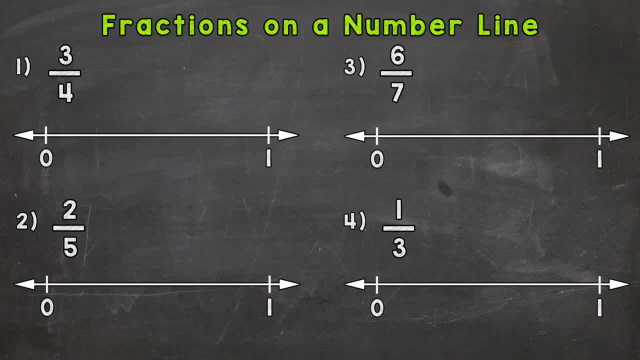 Welcome to Math with Mr J. In this video, I'm going to cover how to place fractions on a number line, And we have four examples that we're going to go through together in order to get this down. So let's jump right into number one, where we have three-fourths. 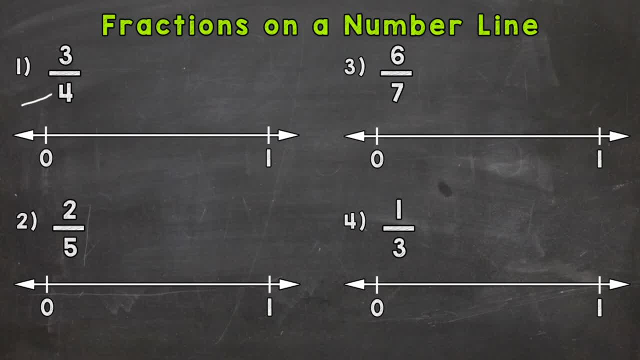 And the first thing we want to take a look at is the denominator. In this case, we have a four, So that means we need to split our number line into four equal pieces or fourths. We're going to be working with the section of the number line between zero and one. 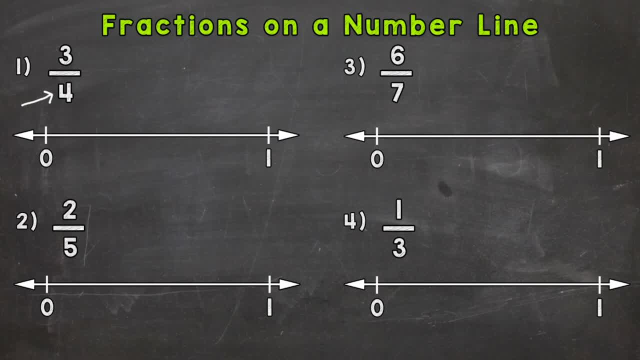 because that's where three-fourths is going to be. So let's split into fourths, And we can do that by cutting in half and then cutting the halves in half, And we end up with fourths, or four equal pieces. 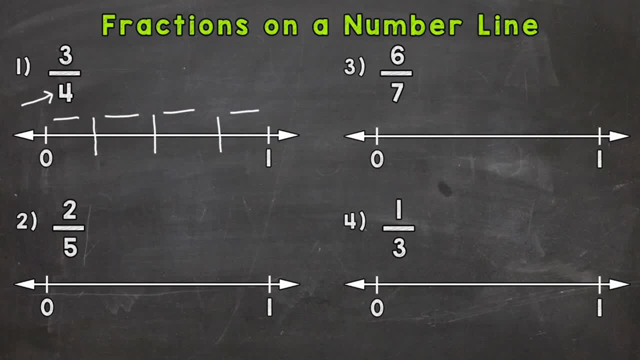 One piece, two pieces, three pieces and four pieces. So our first mark is one-fourth, Then we have two-fourths or a half, if it was simplified- Three-fourths, and then four-fourths, which is equal to one whole. 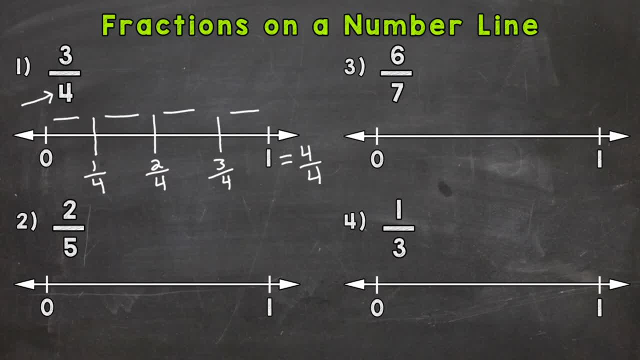 Whenever you have the same number as your numerator and denominator, it equals one whole. So we have everything marked on our number line. Then we need to find three-fourths, which is right here, And we are good to go with number one. 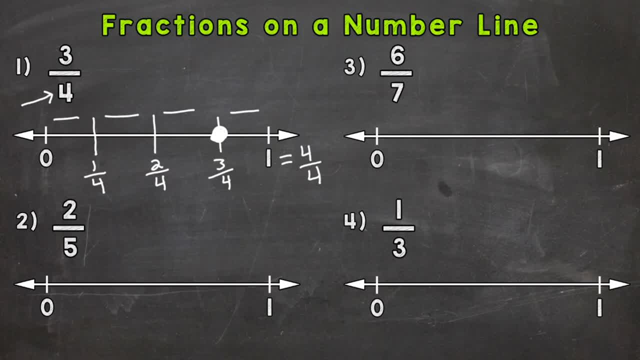 So on to number two, where we have two-fifths. So our denominator of five tells us that we need five equal pieces or fifths. So one-fourth, One, two, three, four and five. Now, with practice- and the more you do, you'll get better with your spacing as far as splitting number lines into fractions. 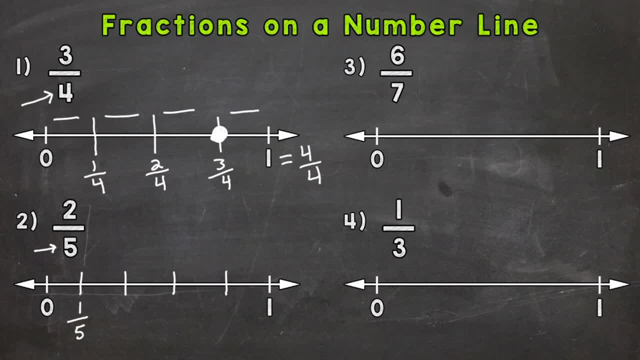 So our first mark is one-fifth, Then we have two-fifths, three-fifths, four-fifths and then five-fifths would be that one whole. So two-fifths would be right here. On to number three, where we have six-sevenths.